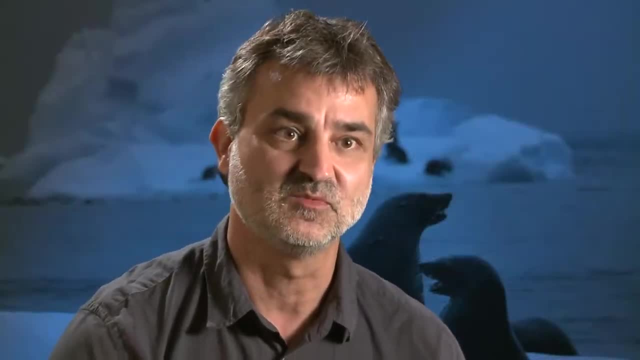 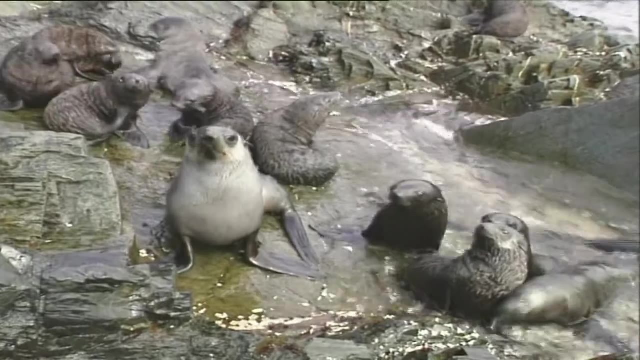 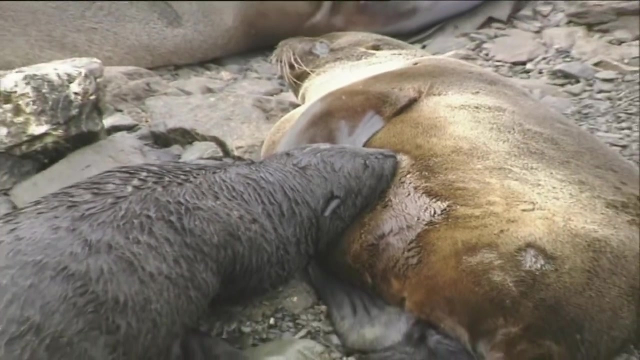 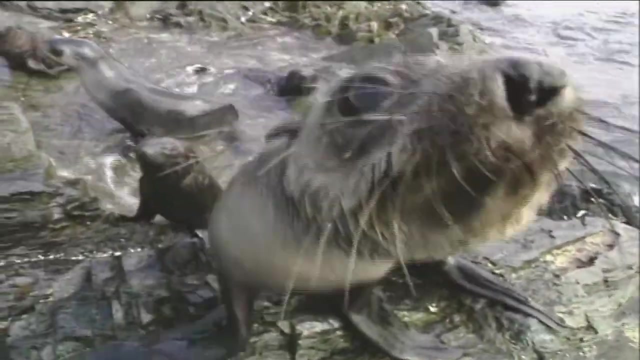 analyzing those data, what is bringing down the population of fur seals and, if that is a problem, that is affecting the entire ecosystem, Amongst those pups that were born, only those that had a bigger mass, bigger body weight would reach the breeding age. And of those that would reach the breeding age, only the 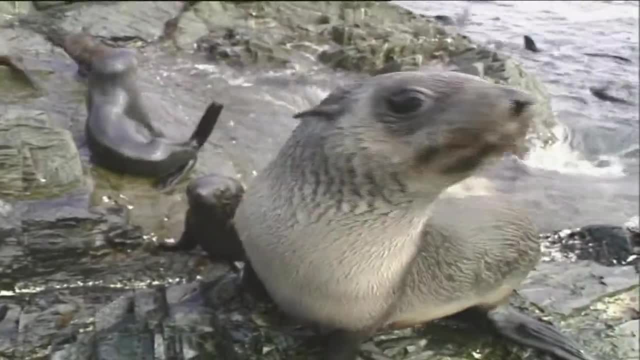 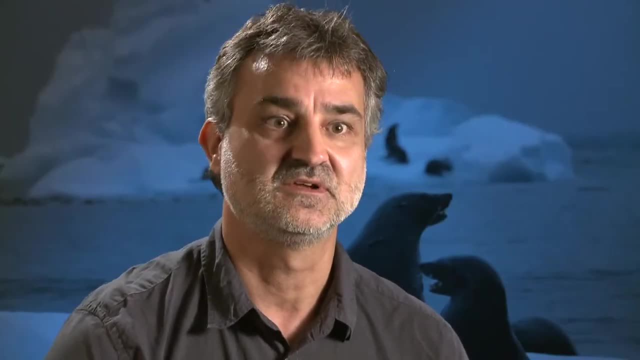 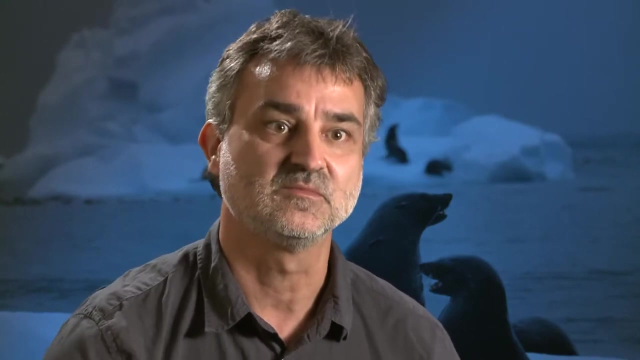 biggest ones for their age, compared to 20 years ago, were the ones that were effectively breeding, And so that was a first result that was consistent with a lack of food in the system, but not an inter-annual food, Inter-annual lack of food between year to year, but a long-term lack of food. So in 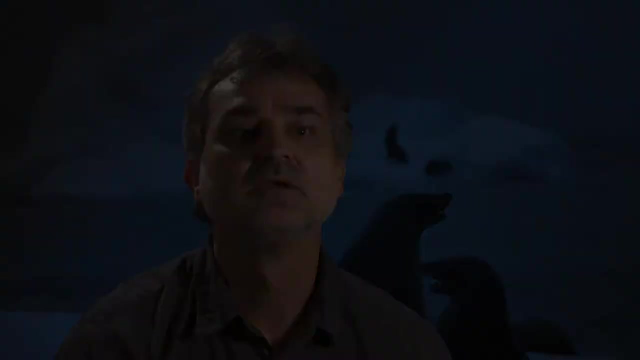 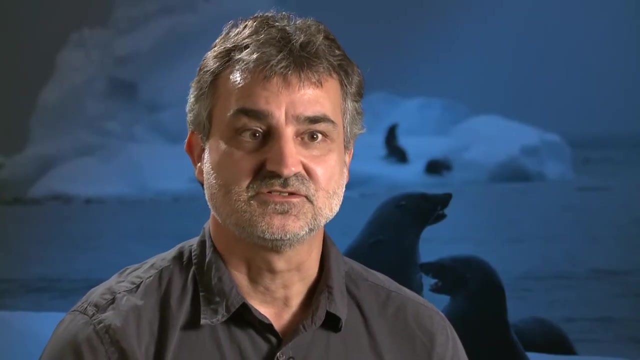 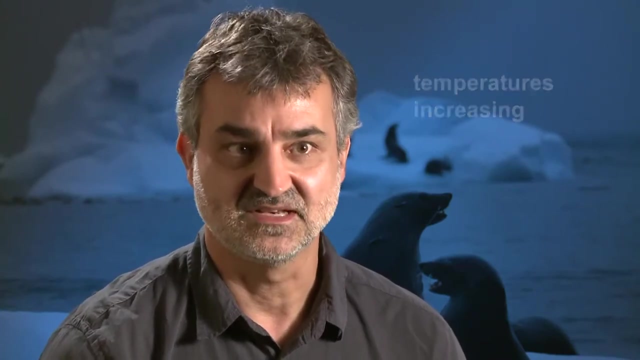 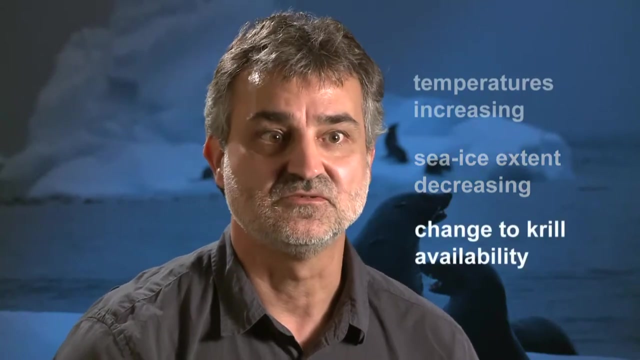 other words, the fur seals were showing food stress. Climate has been changing on South Georgia since the 1990s very rapidly. Temperatures both of the air and the ocean have been increasing and the sea ice extent further south has been decreasing, And all has been related to a change in the availability. 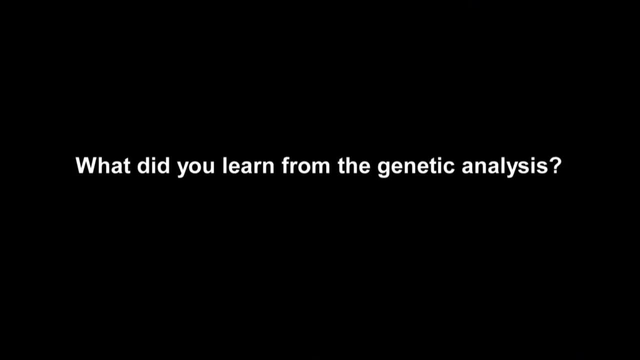 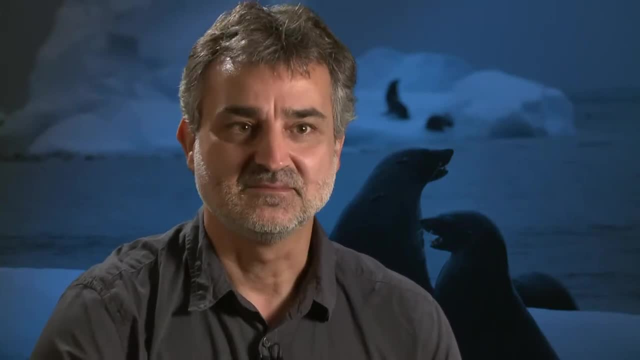 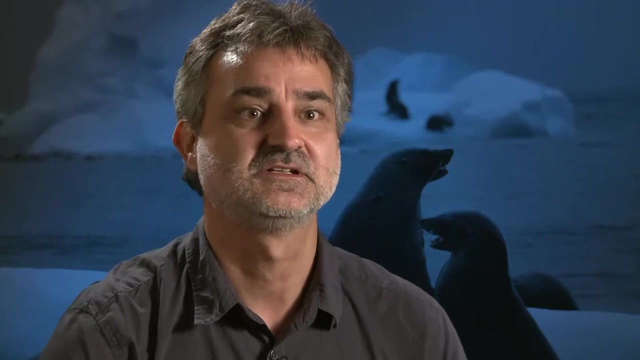 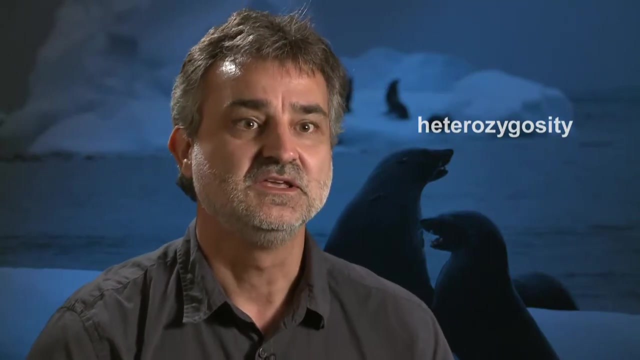 of food. We found that there has been an amazing change- very unprecedented- in the heterozygosity of Antarctic fur seals. Let me explain what heterozygosity is, because it may be a bit of a difficult term for many people. You get one strand of DNA from your mother and you get one strand. 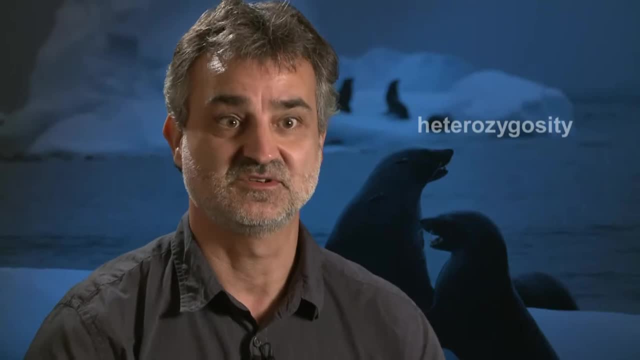 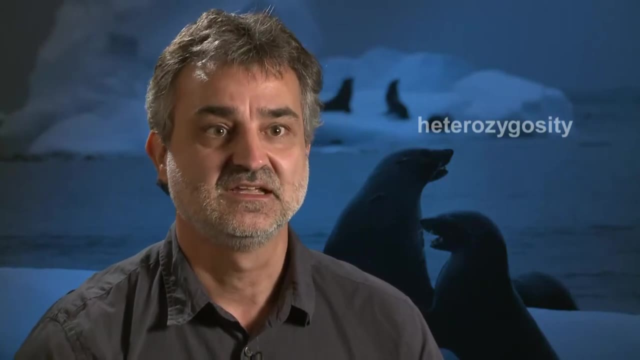 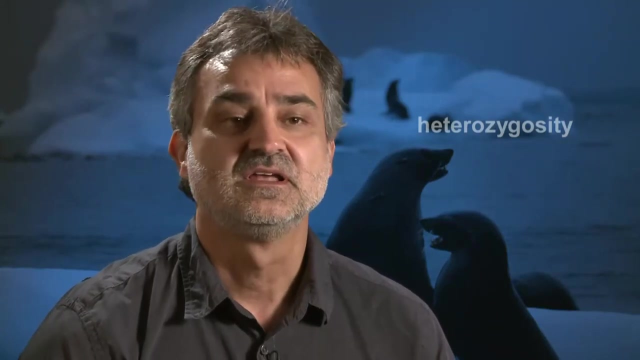 of DNA from your father. You get one strand of DNA from your dad if you are a sexually reproducing organism, like humans, like dogs, like flies. And along those strands of DNA there are points between each one, each other that are the same and points that are different, So the more different. 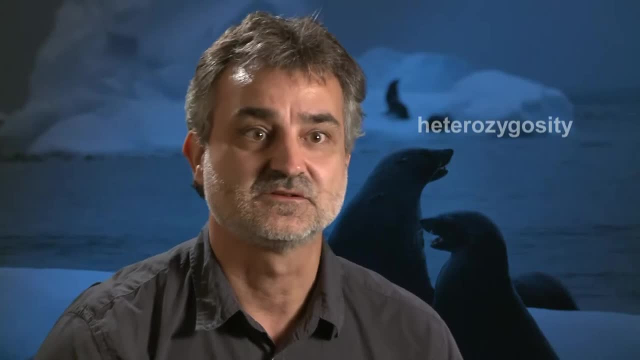 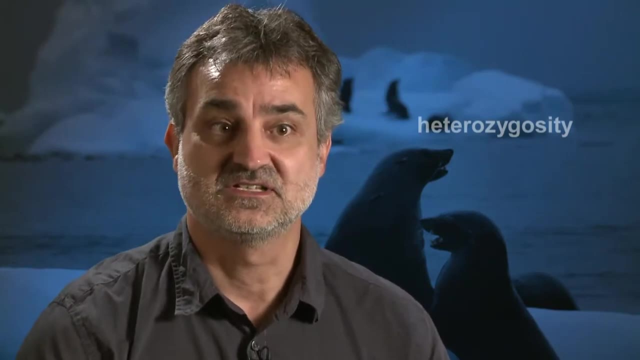 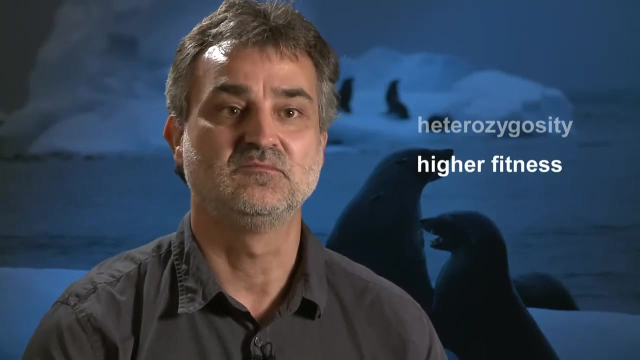 that are those strands of DNA, the more heterozygos is an individual, And heterozygosity, which is the characteristic of being heterozygous, has been associated with higher fitness. Fitness in the sense that you are more able to survive and you are more able to reproduce successfully.